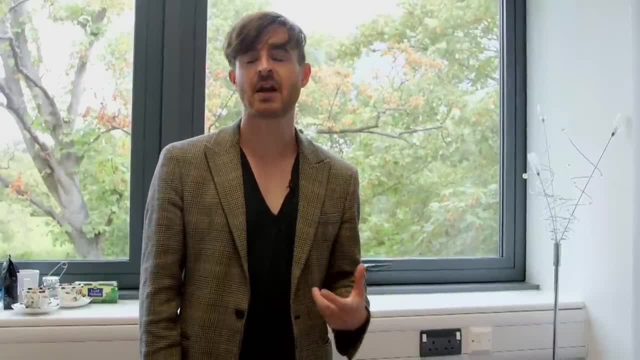 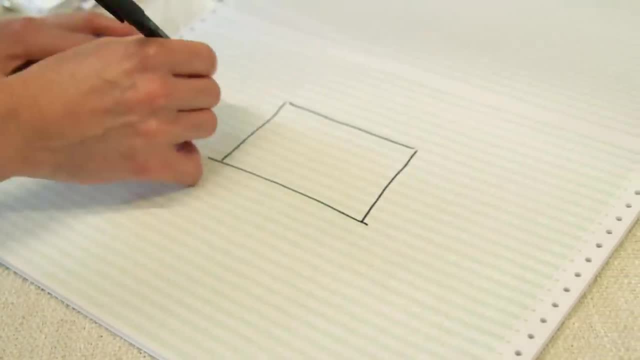 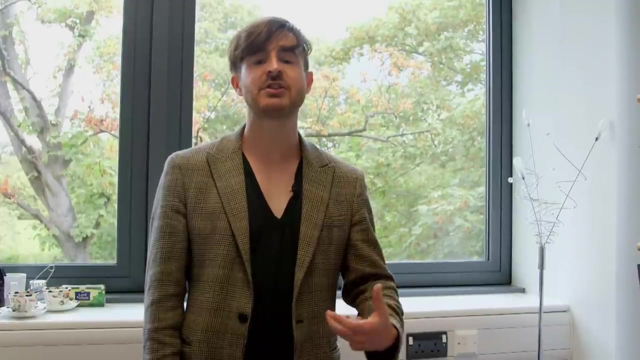 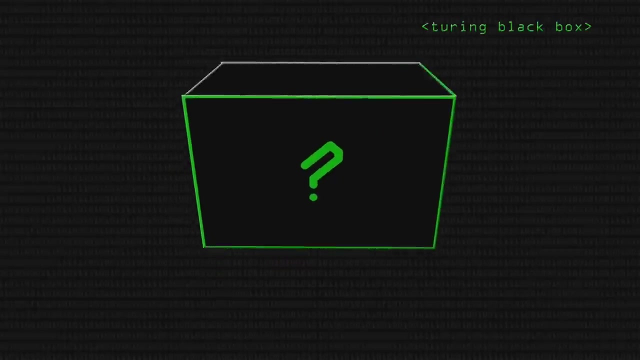 with a brilliant solution. His idea goes something like this: Suppose we have a program and let's just draw it as a black box. It's going to take some inputs and it's going to give us some outputs. Our program is going to solve some problem, A problem like: do the premises entail the conclusion? We ask it. 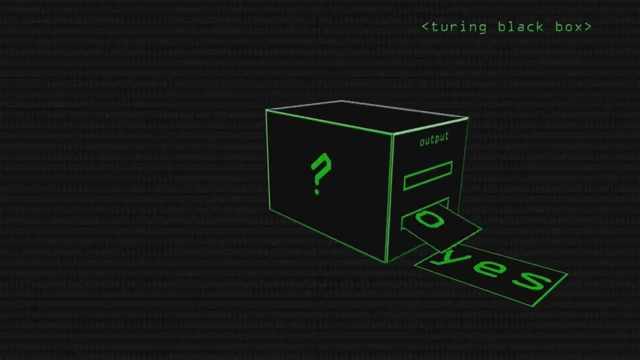 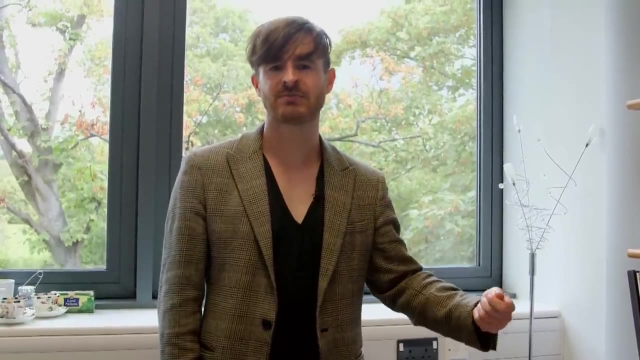 a question and it will give us an answer: yes or no. Now here's another question we can ask. Let's look at all of those possible programs, and we're just thinking of them as black boxes at the moment. We might want to know is this: 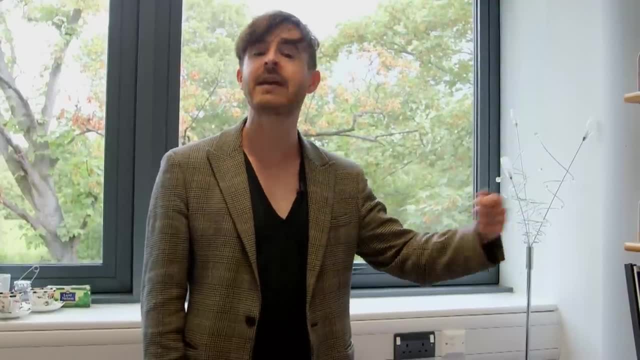 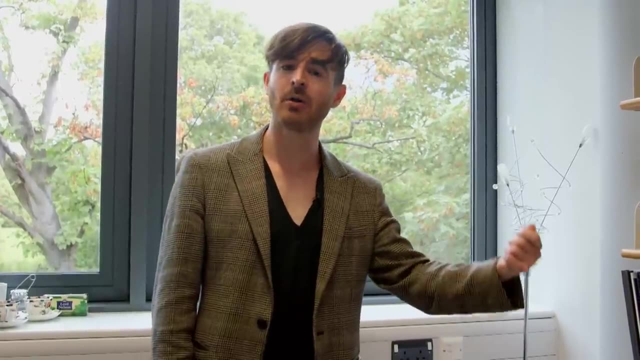 program, given a certain input, going to give us an answer, or is it going to trundle on forever and never give us an answer? That is, is it going to halt or is it not going to halt eventually? So think about your computer running. You want it. 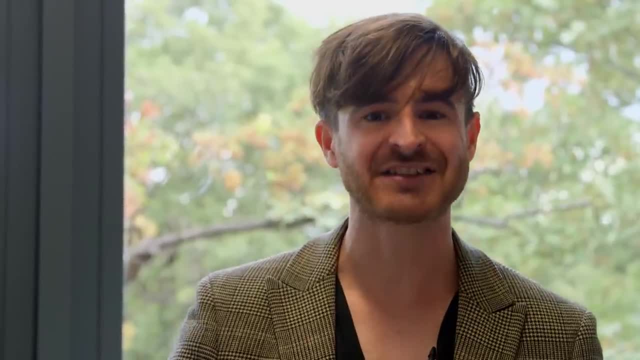 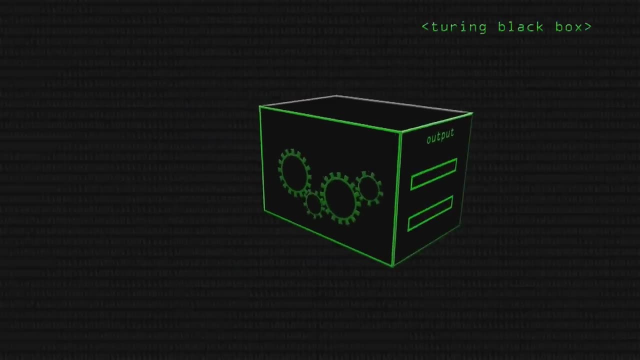 to give you an answer, and whether it's a good answer or a bad answer, it's better than no answer. No answer would mean the computer trundles round forever and ever in a loop, and you would just never know whether it's going to finish today. 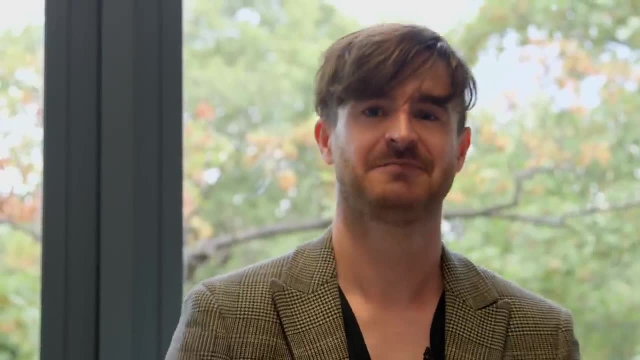 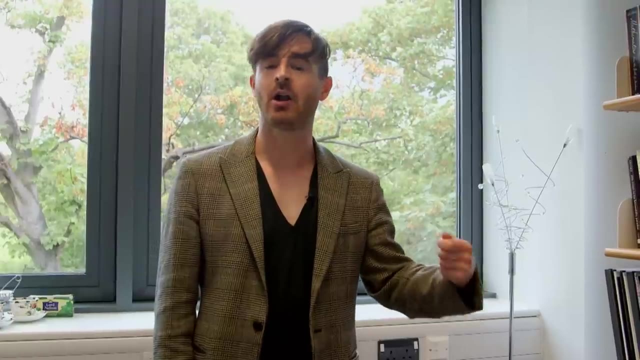 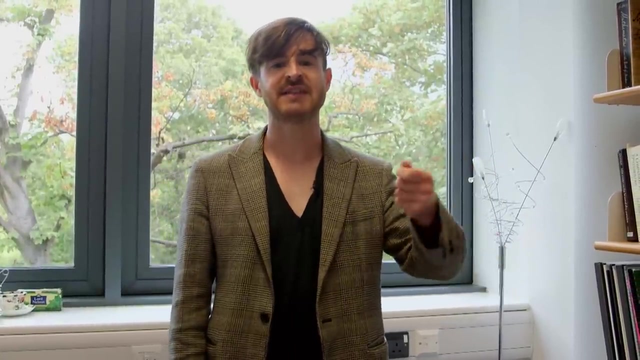 tomorrow or the day after, So halting is good. So there's another question we can ask: Given some program and some inputs, will it ever halt? Now it turns out that our logical problem- do these premises entail this conclusion is very similar to this. 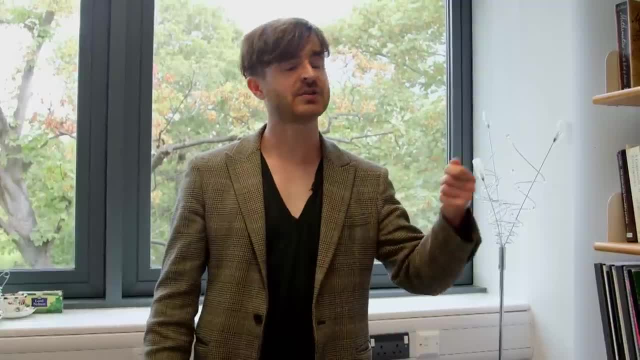 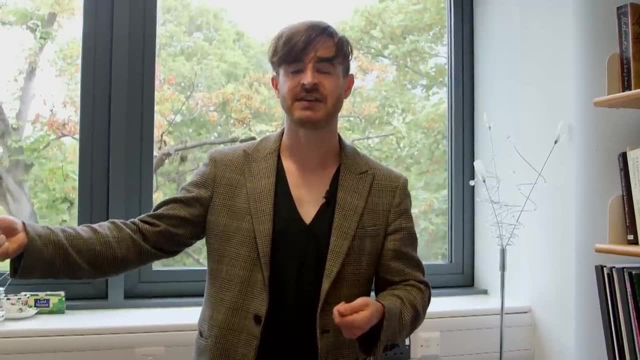 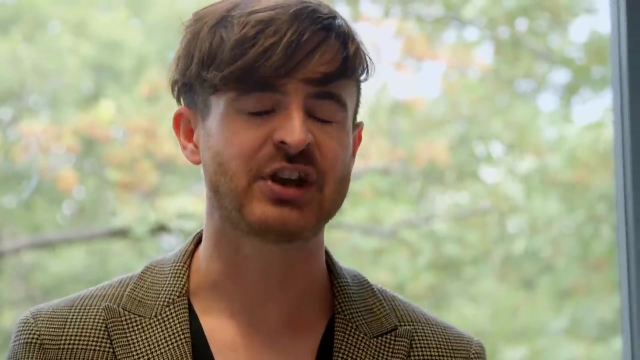 halting problem. In fact, if we can solve the logical problem, then we can solve the halting problem. Will this program halt on this input? So the clever part of Turing's proof is to show that it's impossible for any machine, however clever it is, to solve the halting problem. 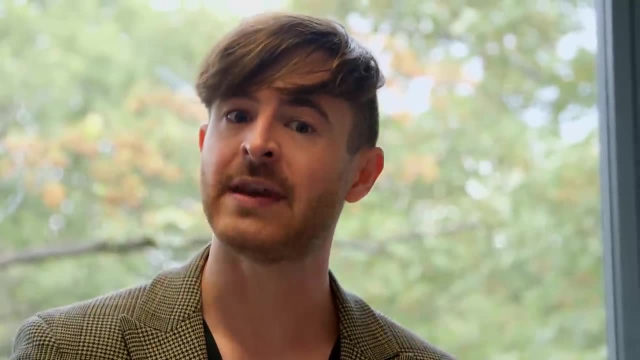 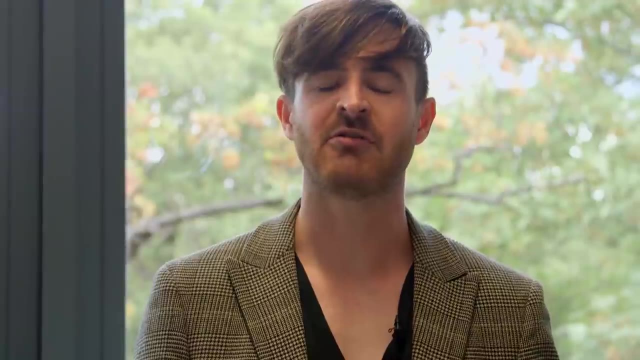 That is, to tell us whether a given machine with a given input will halt or not. And here's how we did it. Let's suppose we've got a machine or a program that solves the problem for us. It solves the halting problem. 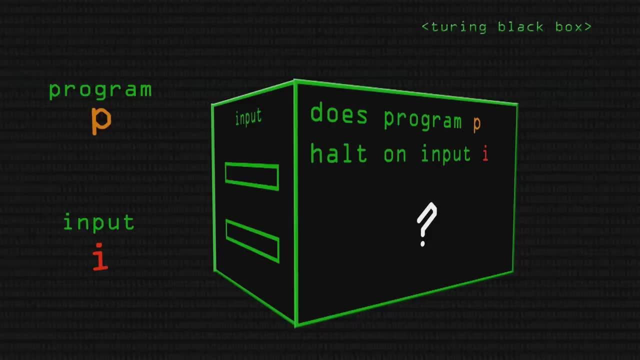 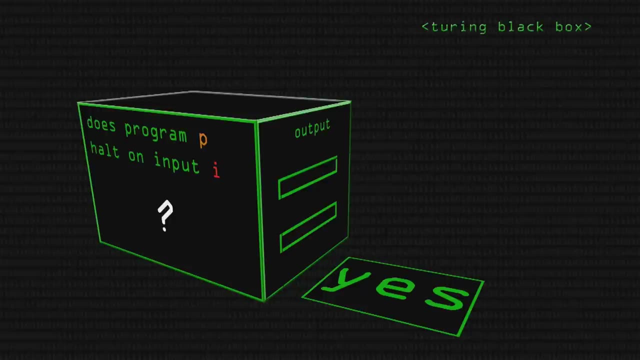 Don't worry about how it works. Let's just think of it as a black box, taking a description of a machine and an input and giving us an answer- Yes it will halt, or no it won't halt. Just suppose that's possible. 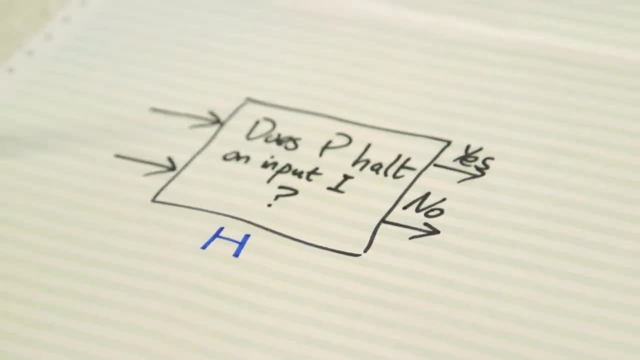 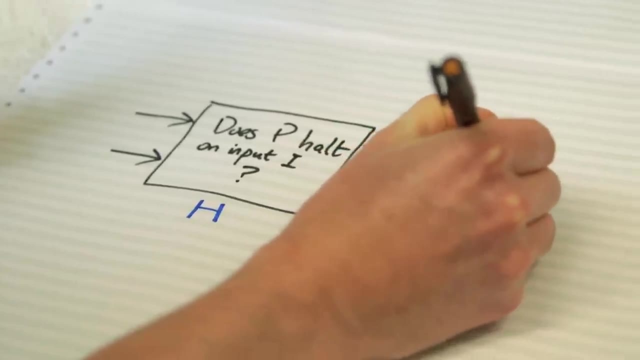 Call that machine H for the halting problem. If you give me that machine, I can transform it into a different machine like this: I stick some extra bits on it so that if it gives me a yes answer, I make it loop forever without ever stopping. 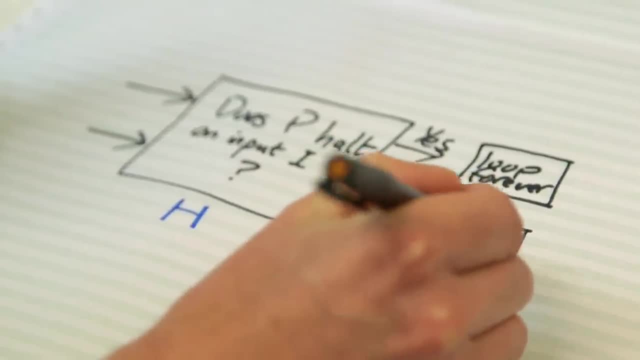 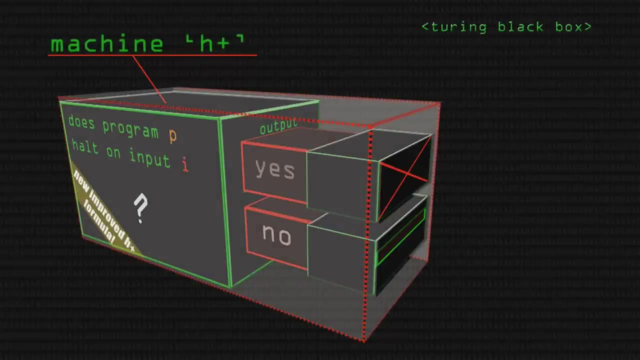 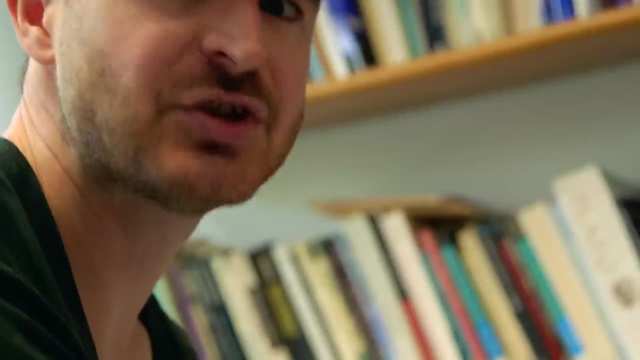 If it gives me a no answer, on the other hand, it's gonna halt straight away. Let's call that big machine, the whole thing, H+. Now here's another question we can ask What happens if I feed the whole machine into itself. 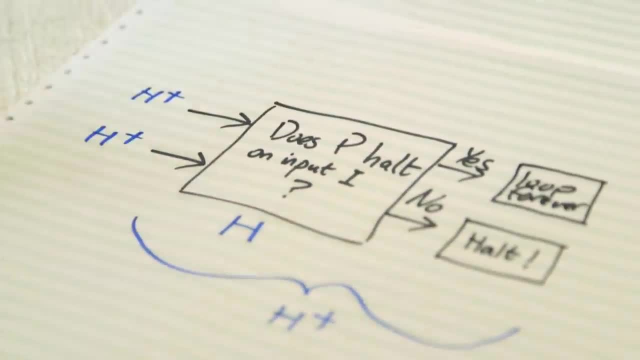 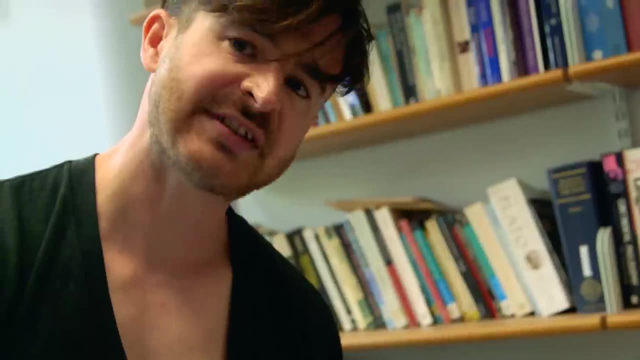 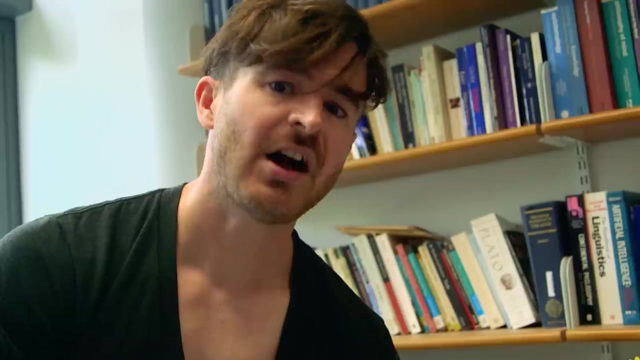 So I'm gonna put H plus in here and H plus in here. So the question I'm now asking is: I'm feeding H plus into itself. So I'm asking the question: does H plus halt given input H plus? And here's where it all goes wrong. 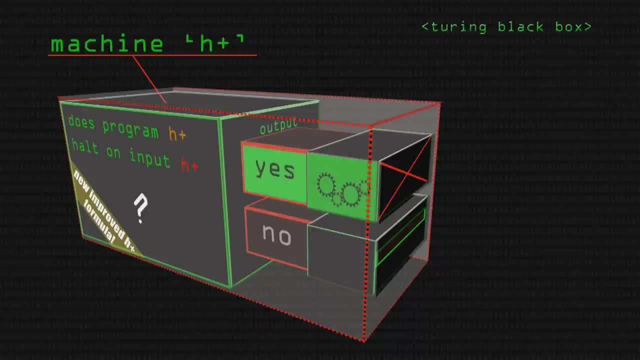 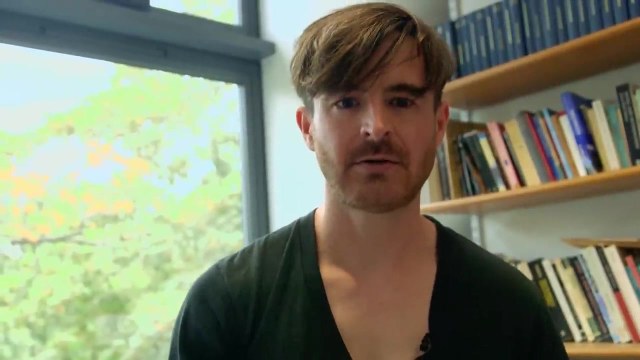 Because if H plus does halt, we get a yes answer, but then it loops forever, so it doesn't halt. On the other hand, if it doesn't halt, we get a no answer, but then it halts. So if it does halt, then it doesn't halt. 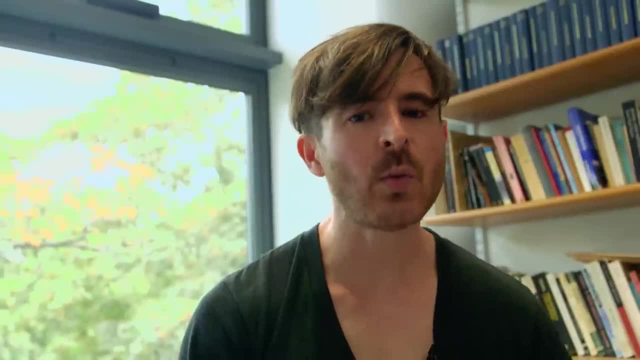 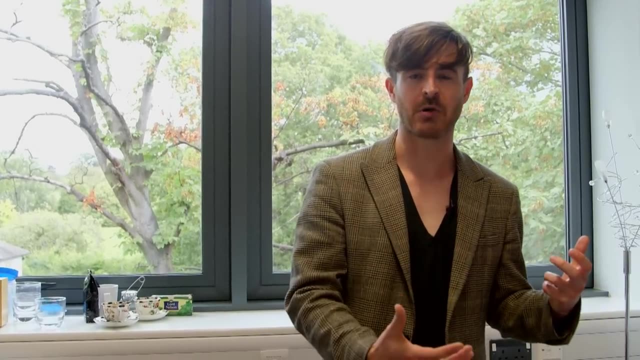 But if it doesn't halt, then it does halt. So the way we get a contradiction, it's a paradox, And what that shows is we started off assuming that we can solve the problem. We've ended up with a paradox, So our assumption was bad. 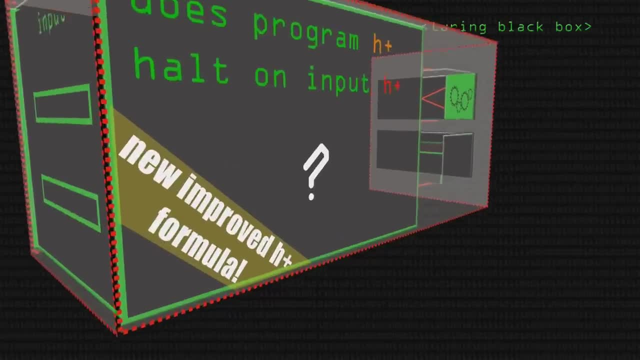 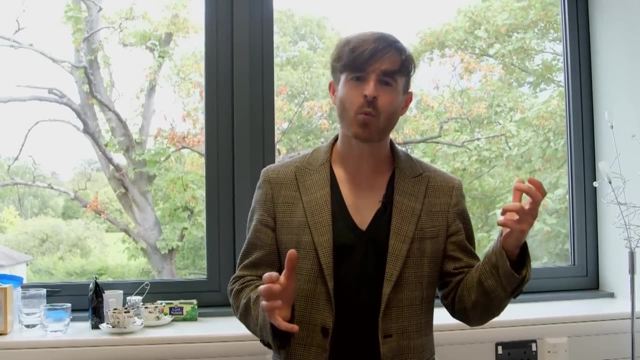 It turns out there's no possible machine, no possible program that solves the halting problem. The really clever bit about Turing's idea is: it doesn't matter what kind of program or machine is, It doesn't matter whether it's an abstract algorithm. 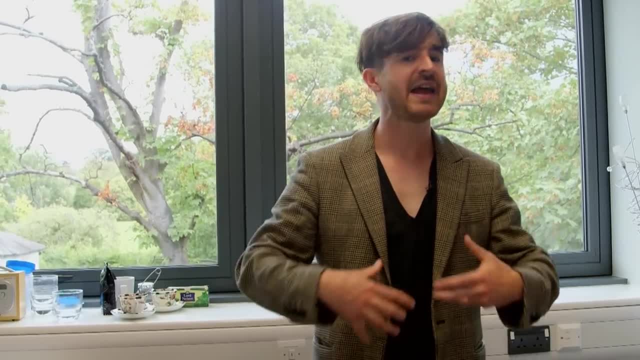 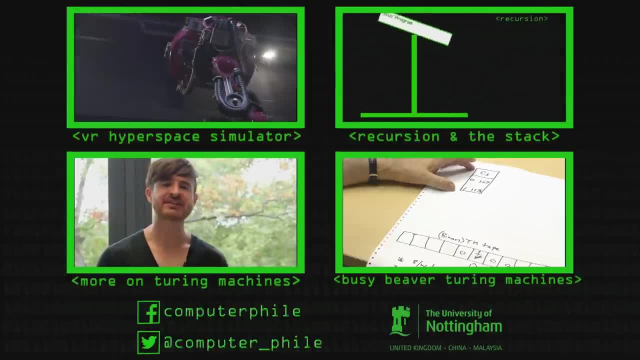 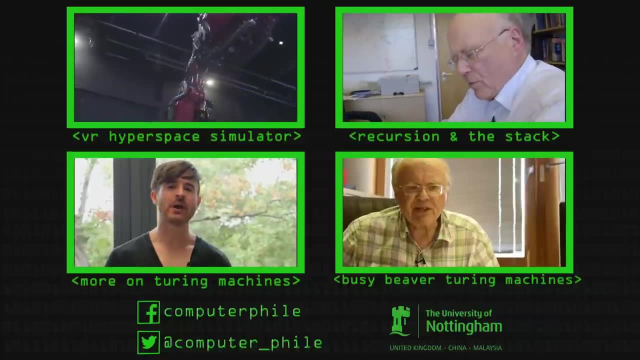 Turing, as part of his argument, had to say a little bit about what's going on in these black boxes, And the idea is that every card represents an instruction in this Turing sheet.